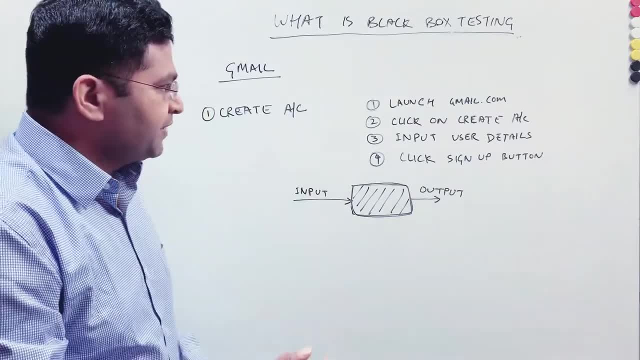 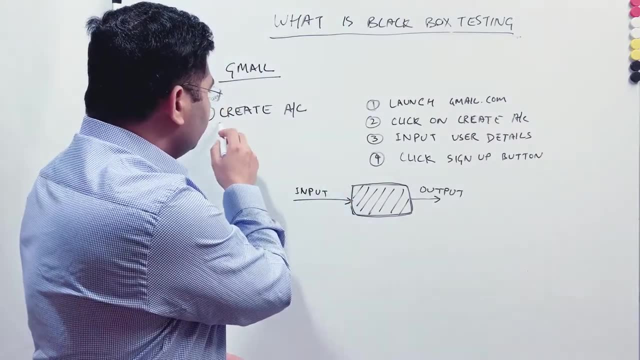 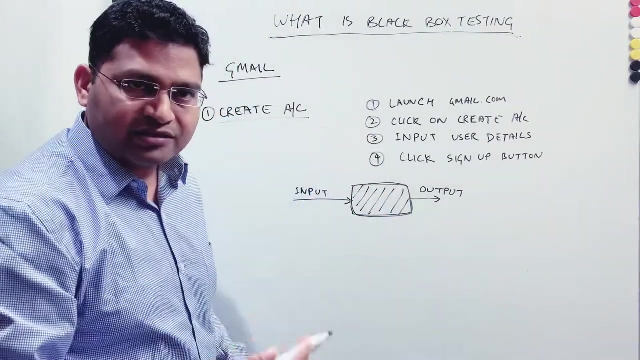 it is the black box for the software tester. So let me take same example that we took in the previous tutorial. So functional test of this Gmail create account feature, Right. So in the create account feature, what we did. if you are testing the create account usually. 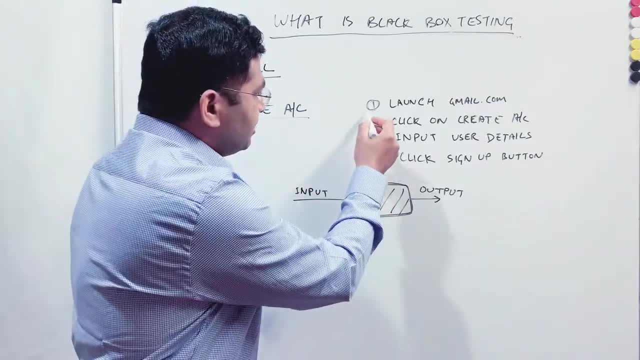 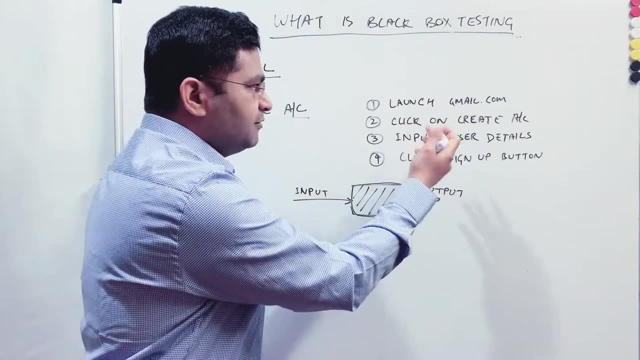 you will follow certain steps, which will be a test case. So here there are a couple of tests that I have written, So I'll launch the application. If I'm testing that particular application, I'll launch that application. you know, in some browser, Right? So in browser. 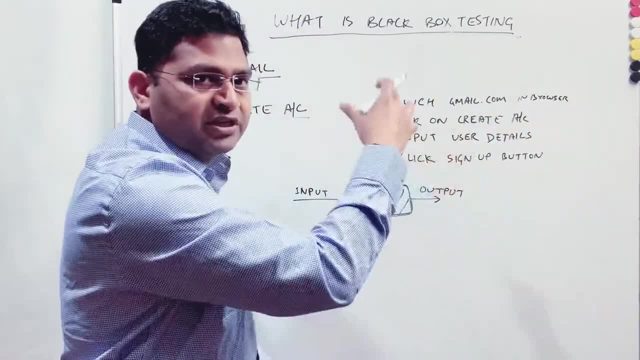 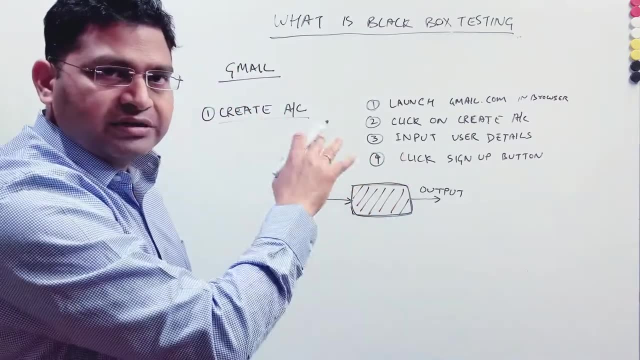 And browser could be, you know, like Chrome, Firefox. So that will be specific in the test cases when you detail this out in your test case, Right? This is just to explain you the steps, So that is why I have not written all the details in this particular scenario. 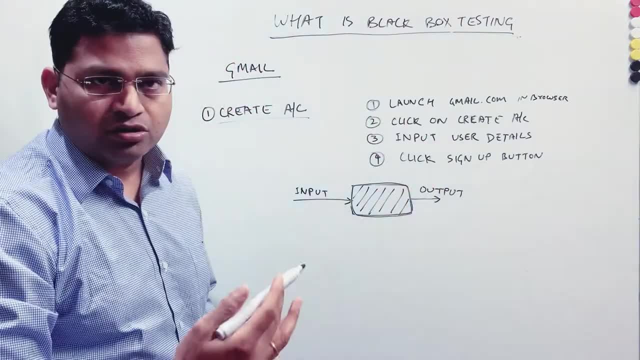 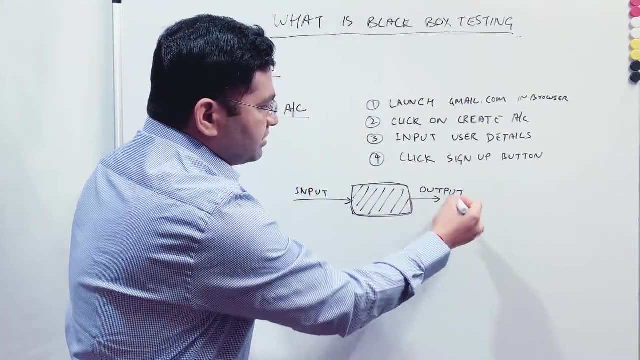 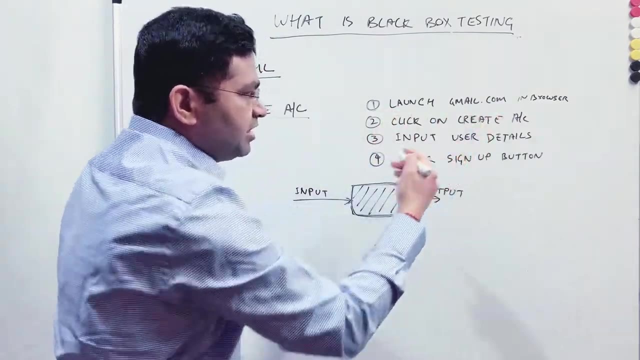 So first step will be to launch gmailcom in the browser. If the launch is being successful, then I will say: output is passed Right. So in here input, the step one input is basically launching Gmail in the browser. This is my input, Right? So these are the actions that I'll do. 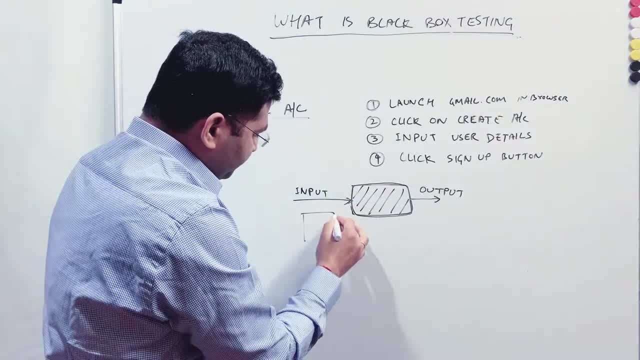 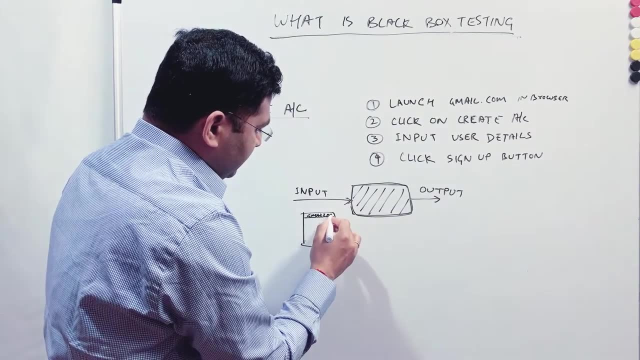 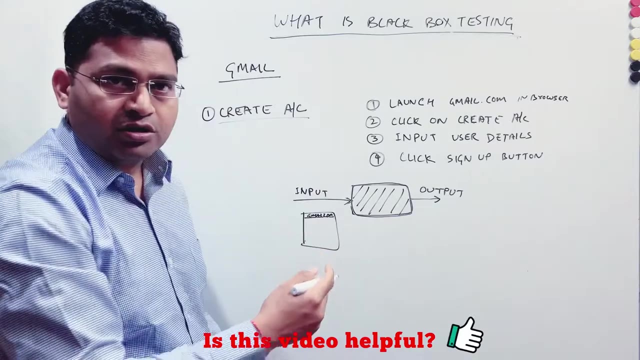 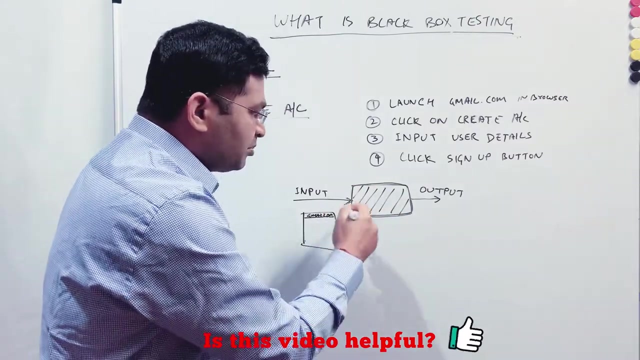 Now, when I open the browser okay, and I type in gmailcom and after typing gmailcom I hit enter right or hit go, then it opens the gmailcom. As a software tester or person launching this application, I don't know what all happens. 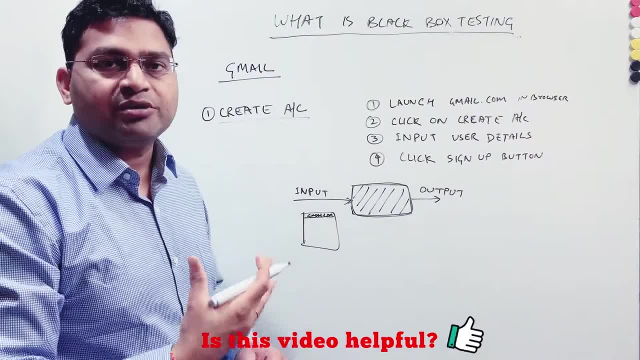 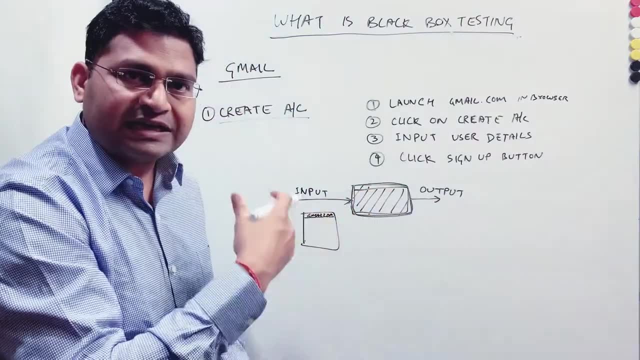 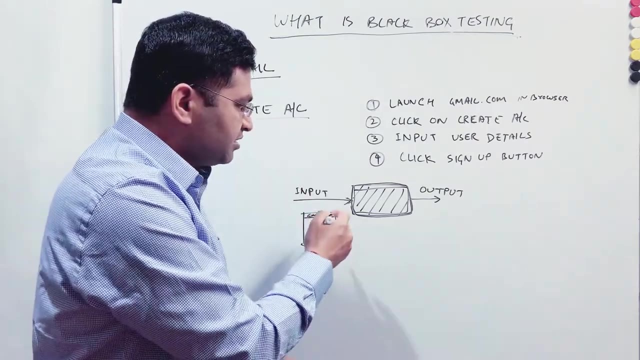 behind the scene before I see gmailcom page on my browser Right. So that is a black box for me. All the functionality. that has happened after I provided gmailcom or gmailcom info in the url and then hit enter. then after that I don't know what has happened. 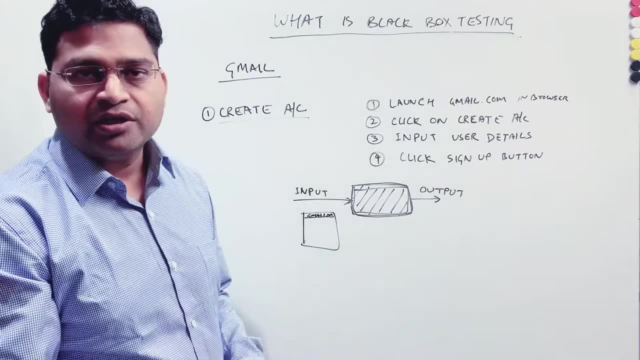 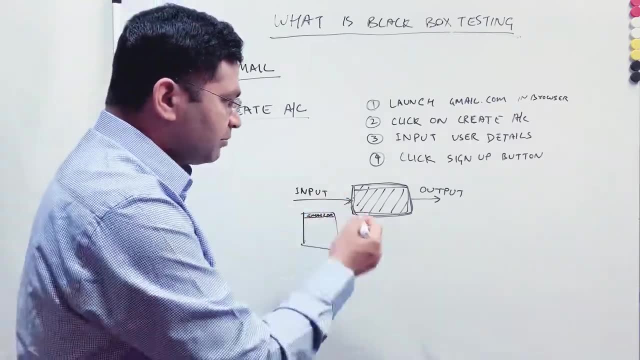 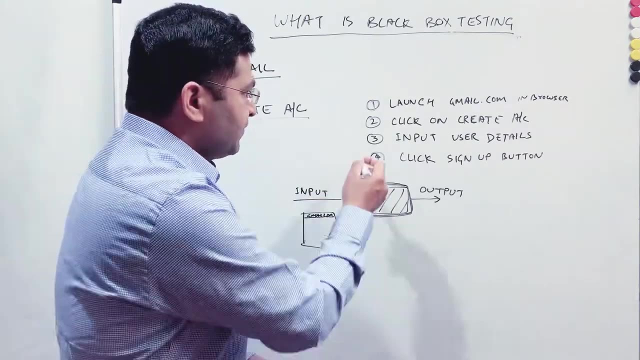 what application implementation is there? what software has been written to basically fetch the data and show the gmailcom page to me? Right? So that is black box for me, and that is why this is the Black Box testing, of how the Black Box testing will work. Second input for me in the same test case is the Group URL. 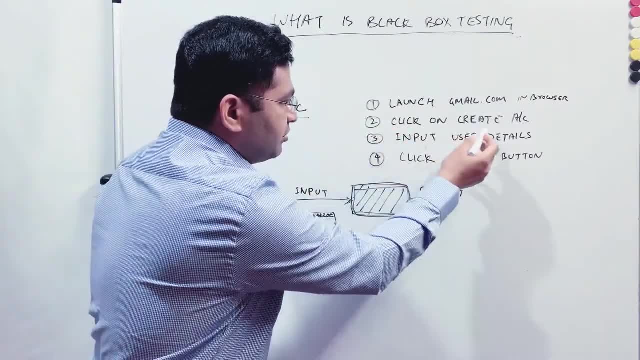 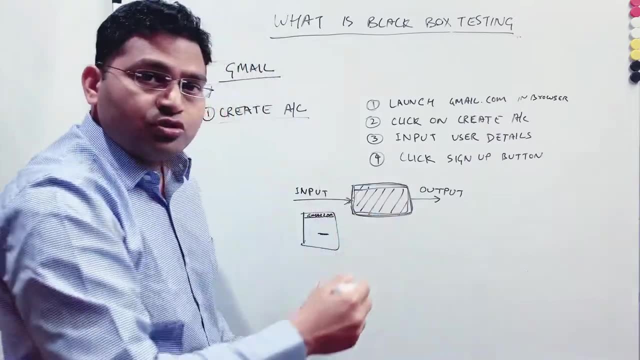 If I come to the dll and click load on their list, right, I'll be able to see it. I will test case: is the black box testing so click on create account. so once I click on create account link, say for example, then I'm not sure what implementation has been done. once a user clicks, 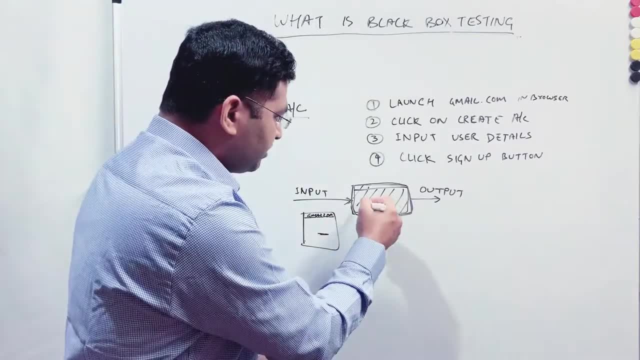 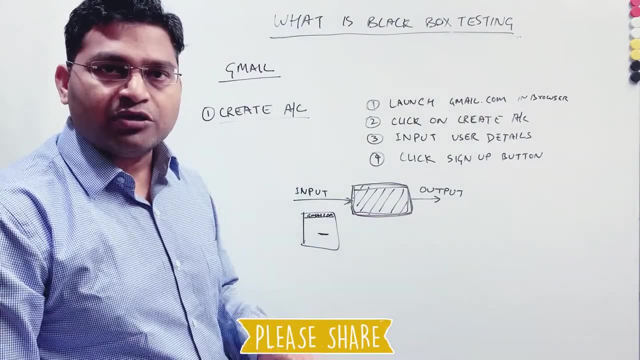 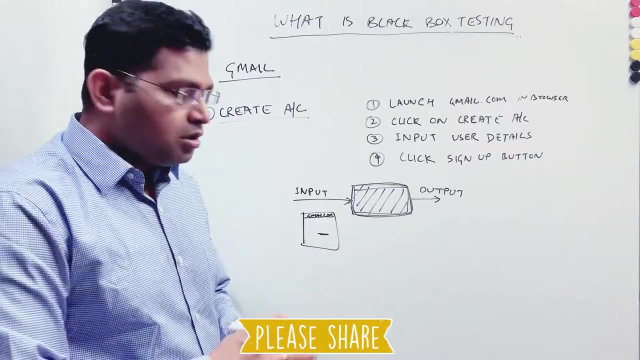 on create account, right. so I don't know what coding is there within this particular box. as an end user, I don't have any idea about it and I'm not concerned about the internal coding, how the methods are written, how the classes are written, how the internal code is being called. 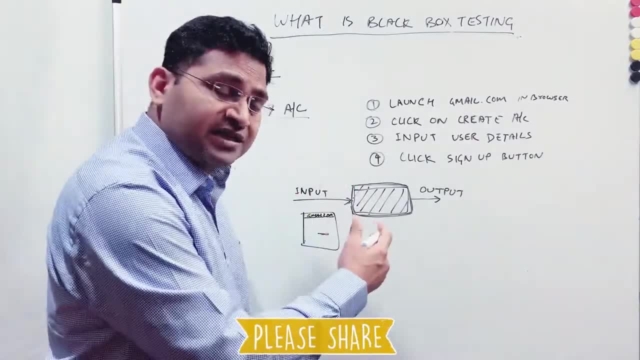 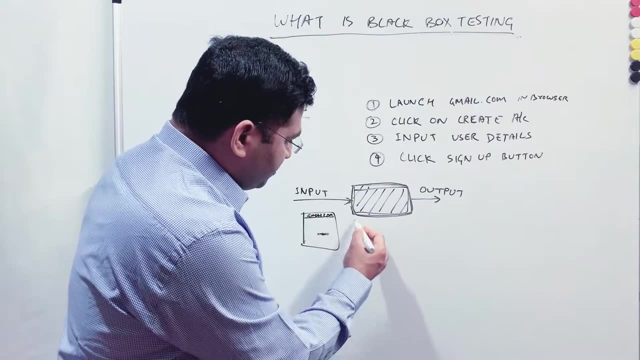 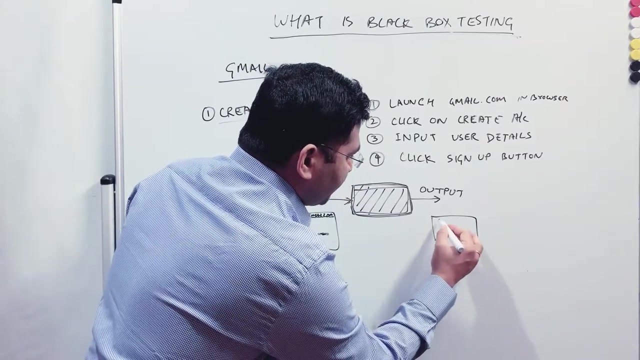 when I click on create account, what all happens inside. I'm just worried about. or I'm just concerned about when I click on create account, you know link I should be displayed, or basically I'll click on, I'll draw here. so output should be, you know, create account, page right, which will have 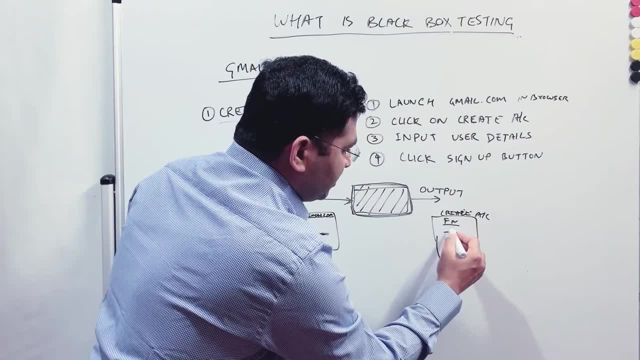 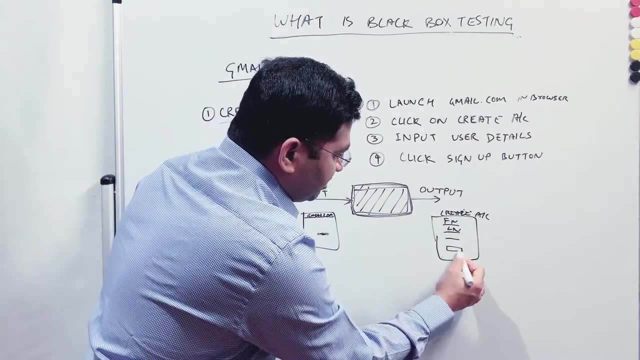 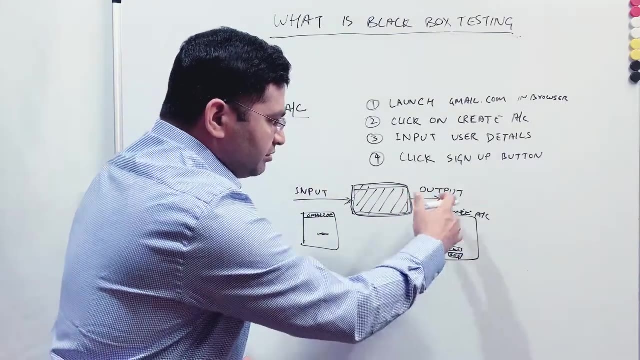 provide your first account, name, last name. so I'll say first name, last name. I'll provide which email. so I have to search the email and then provide the password and then click on register. all right, so I need to verify these details. but internally, when I click on create account, how everything worked or how the 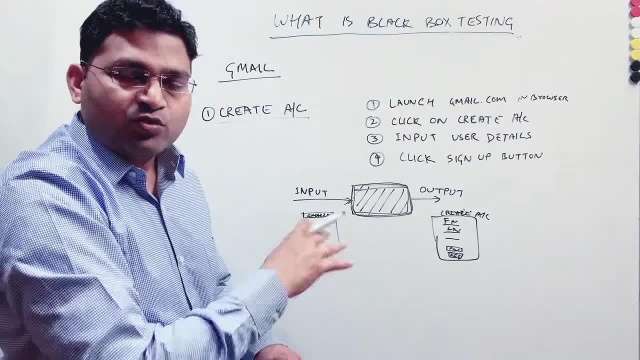 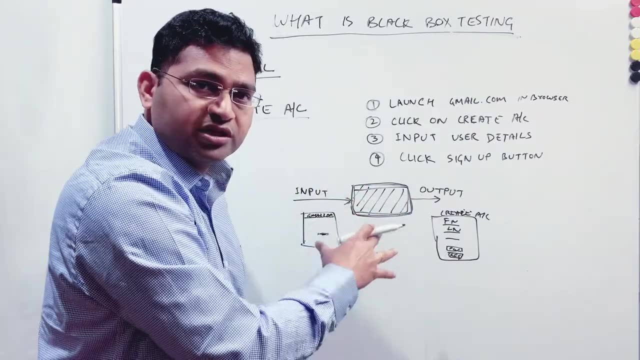 code has run internally as a manual tester, as a, you know, black box tester or black box testing. I'll say first name, last name. so I'll say first name, last name. I'll provide which email, so I have to provide which email. I'm not concerned about any of those internal working details, right? so? 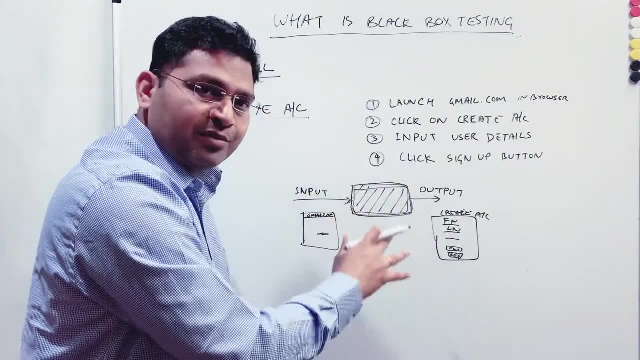 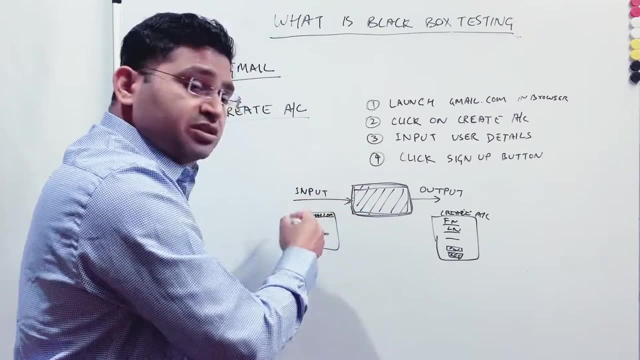 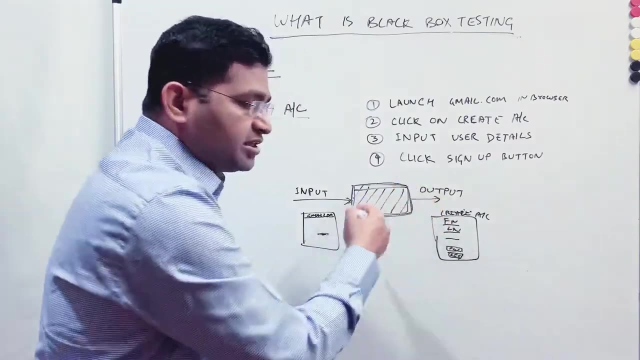 this is how the black box testing will happen and what or what black box testing is. so each step in your test case just is is basically the input, and whatever expected result of your test case is is the output in terms of black box testing. in the third case, I'll provide the input user details. 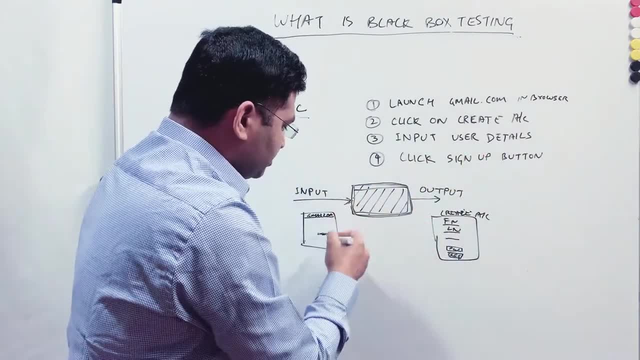 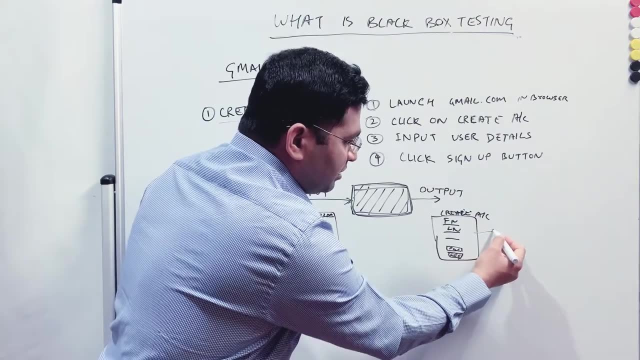 right and then click on sign up button. so once you've done that, you can go to the next step and use the details have been provided here. that becomes the input and a user clicks on you know sign up or register button and then he should be redirected to the. this is the black box in this.